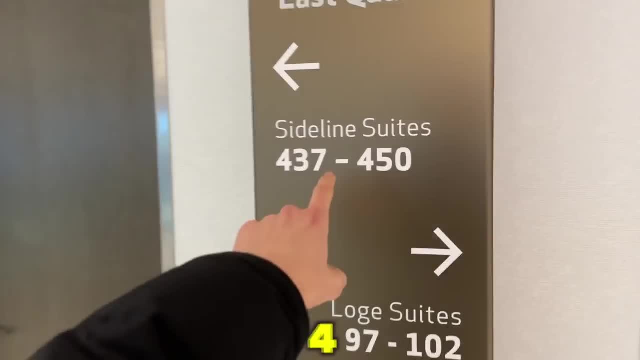 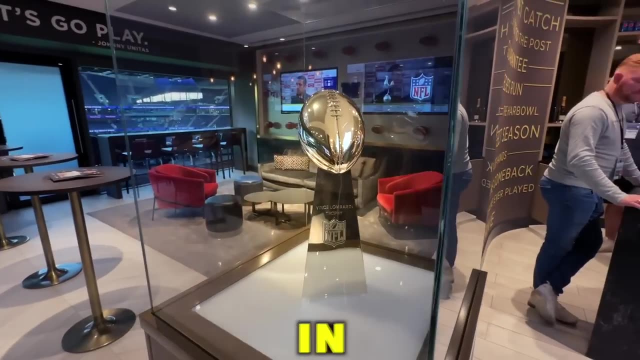 And I will go to the cheapest Premier League seat in the whole league. 4-4-1 is where we're going. We've made it in And, oh my God, is this a hotel? It's massive. They've actually got the NFL trophy. 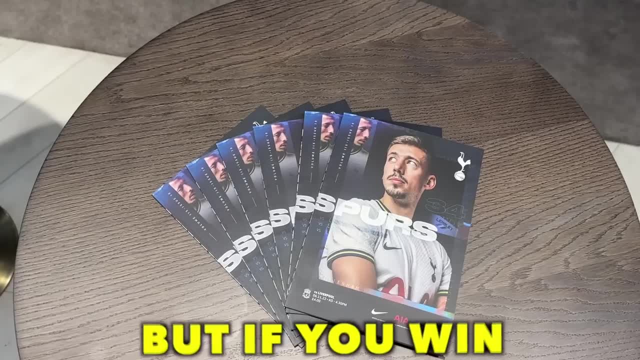 I believe I'm the first one in the box as well. Now, I don't know much about the sport, but if you win the Super Bowl, you win that thing And we're making out to the pitch. Absolutely beautiful, Thoggy boy, take it away. 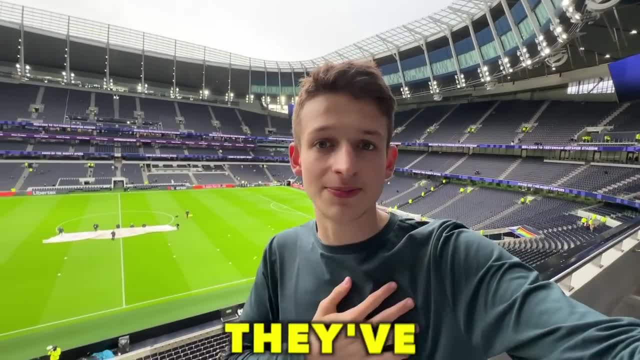 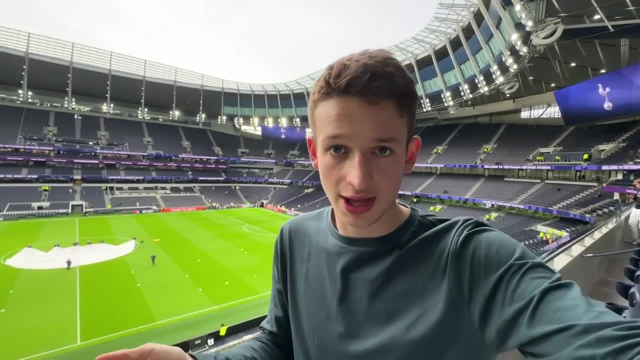 This is one of the best views at a football stadium I've ever had. They spent one billion pounds on the stadium And we're getting to enjoy one of the biggest Premier League football matches this season: Tottenham against Liverpool. My father and I are one of the best seats in the house. 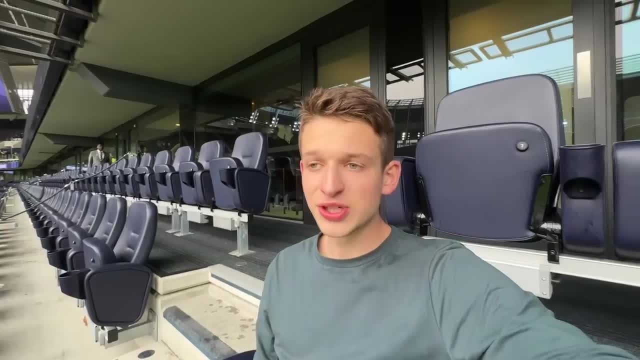 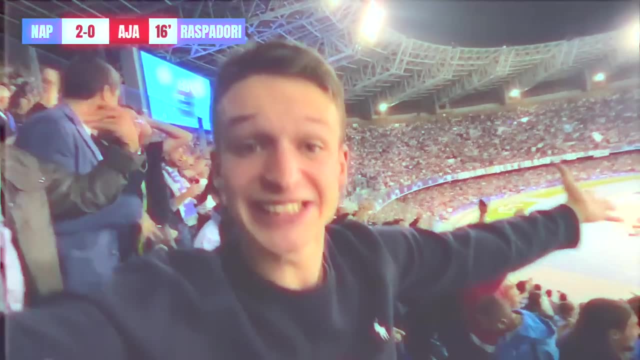 I was amazed. I was the first one here And I got a bit emotional. These opportunities can only happen for you guys. That's why I'm constantly saying thank you. Eight nine years of constant uploading, going to matches all around the world. 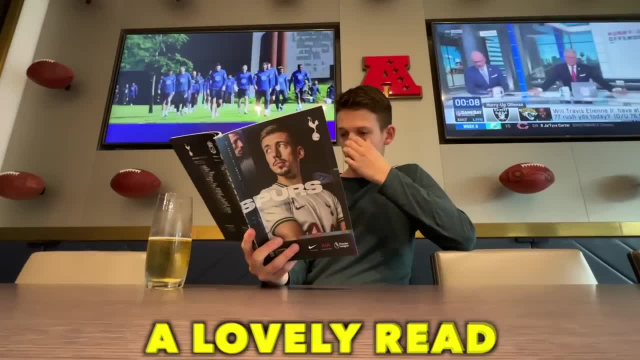 And I get to go to a game like this and watch a match as big as this, And as I was having a lovely read of the Spurs magazine with my beer, an old man turned up. We found a wild thug. Dad, Look at him. 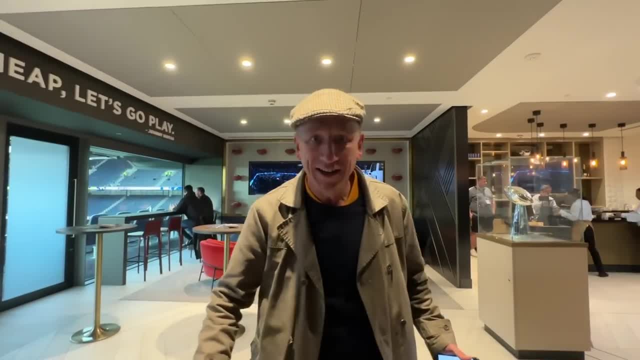 I'll tell you what this is. alright, isn't it, Mate? this is insane. I've got a special hat on today. Who the bloody hell is that? Theo? you come in a flash corporate box. You know what you've got to have. 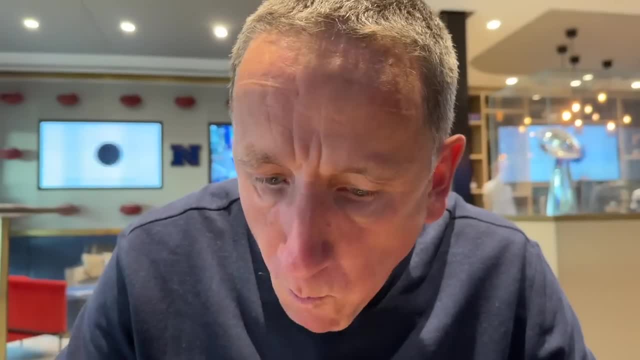 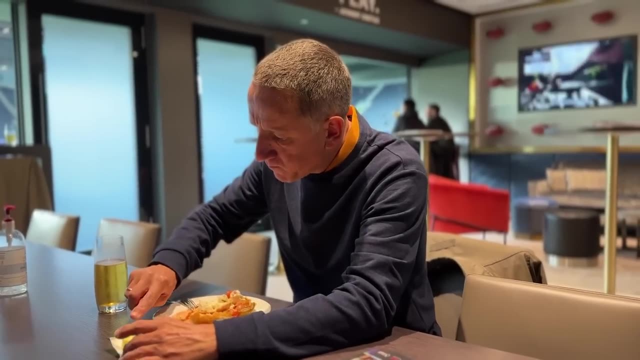 That prawn, Bring it on. I hope you're watching Roy Keane, Just for the running joke. Right right, Dad, Eight out of ten. Dan, the man had just explained to us This was the best box, not only in Tottenham, which is the most expensive stadium in the world. 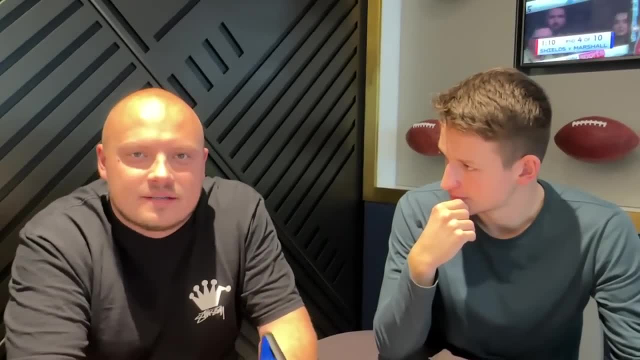 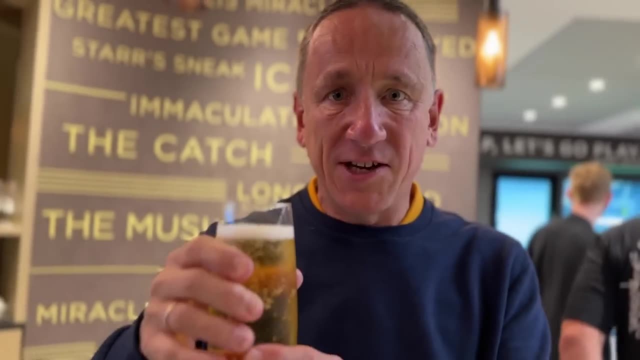 but the best seat in the house, One of the joint biggest, or one of the biggest boxes in the stadium. Time for another beverage. Today I'm going to try a tasty, cold American beer. It's a Budweiser, a classic. and it's NFL day, isn't it, Theo? 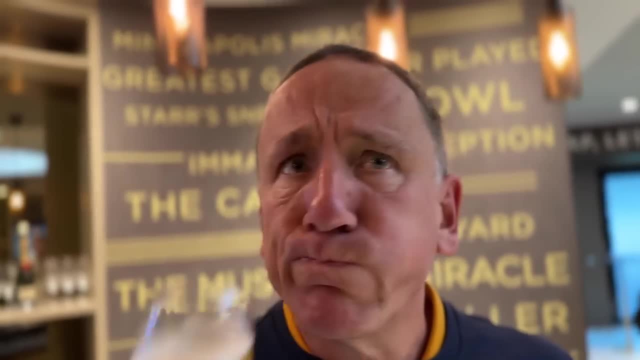 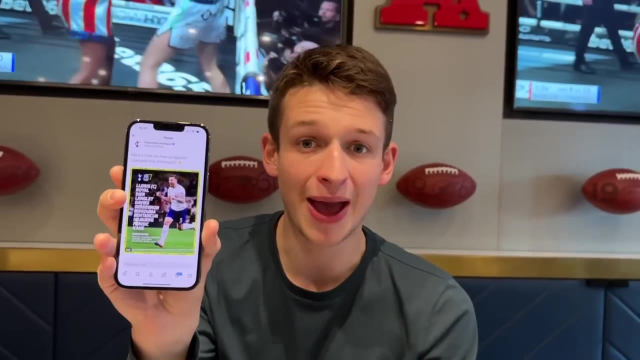 So let's give it a whirl. Come on, Give us the thug Dad Best seat you've ever been in. That is a refreshing change. I'm giving that 7.0.. Decent beer. They're playing Perisic in a 3-5-2.. 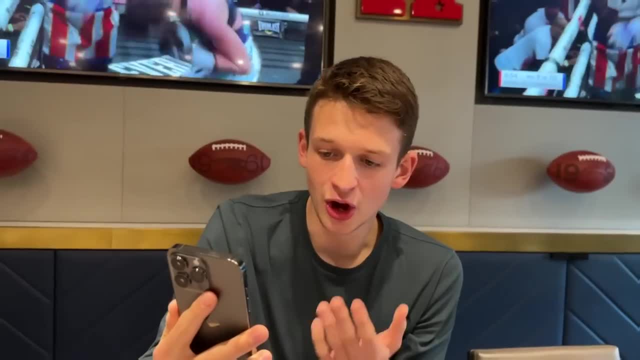 The front two is going to be Kane and Perisic. Antonio Conte has gone bonkers. Firmino Salah, Darwin Nunes, who I expected to drop a masterclass. Do you know what I'm going to say? Liverpool to win 2-1. 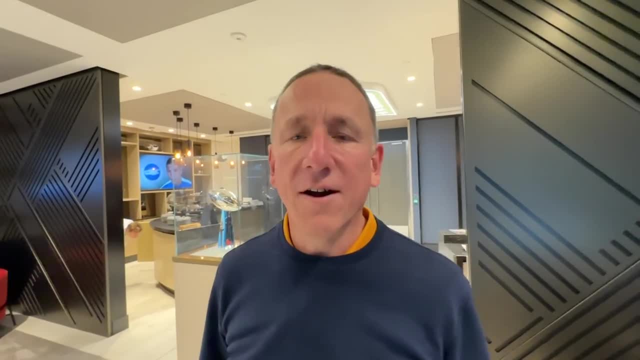 Oh, this is priceless. This is, I don't know, a million quid a year, mate. It's opposite Daniel Levy's box, isn't it? So it's actually bigger than any box you'll find in the stadium, The biggest box in this amazing stadium. 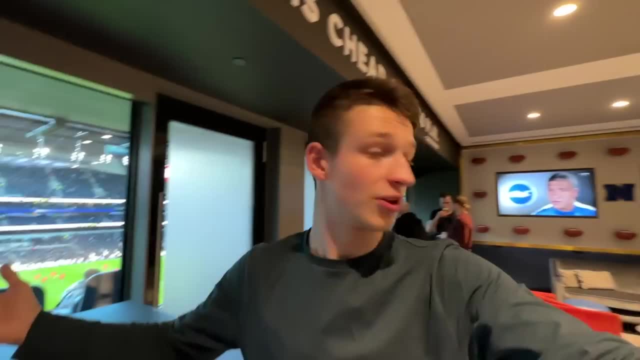 This is what you pay for. You get a limited drink, a limited food. We've had our starters, not the main, Out to see the players warm up and back through for the main course. The mains are out. Let's give it a go. 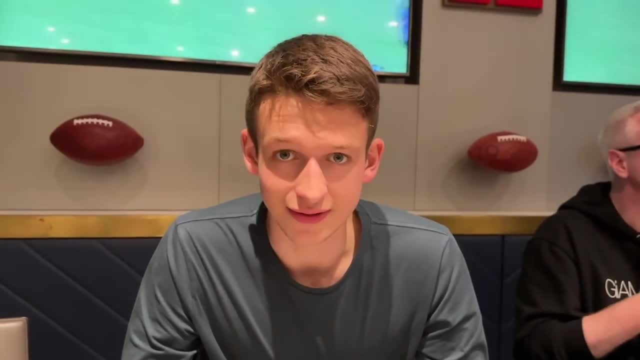 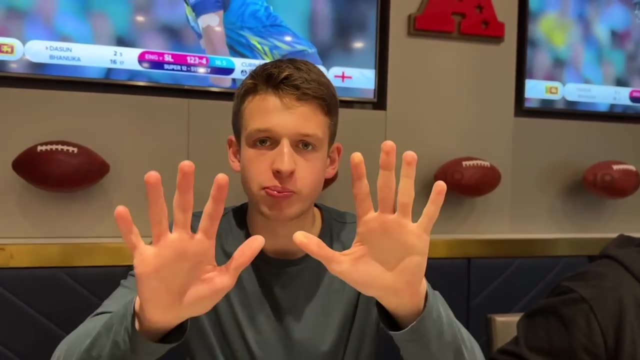 We've got a Sunday roast before Sunday roasted in Tottenham. I don't know where to start. We're going to get straight to the beef. 10 out of 10.. Oh, my goodness, We're not playing well at the moment. 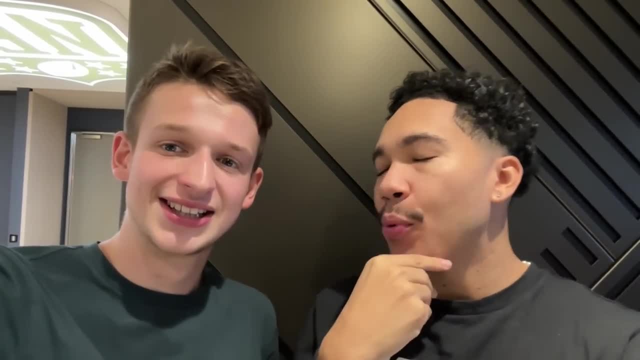 Liverpool aren't playing well, but I don't know. I feel this is the type of game Liverpool will get up for, though We saw that against Man City. I see that, So I'm going to say a draw, hopefully. I'm going to say a draw. 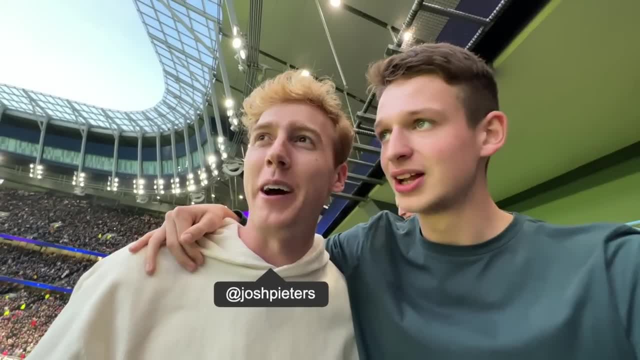 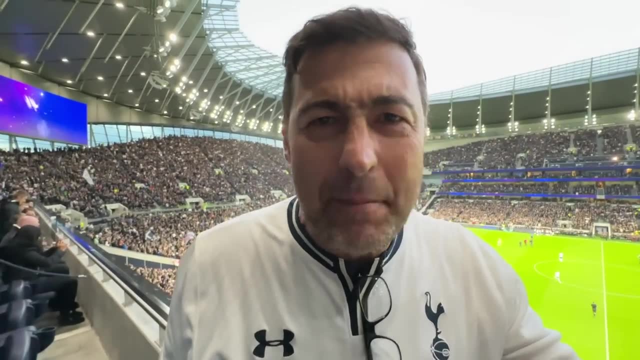 Let's get outside. It's time for kick-off. I've got a prediction for Tottenham to win, but let's go with 1-0 for Tottenham. Just today, For South Africa, 3-2 to the mighty, mighty Spurs. 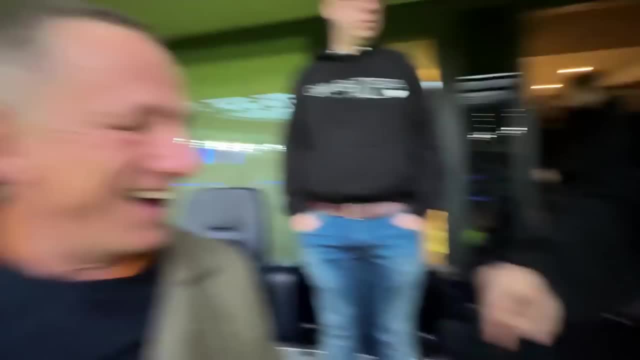 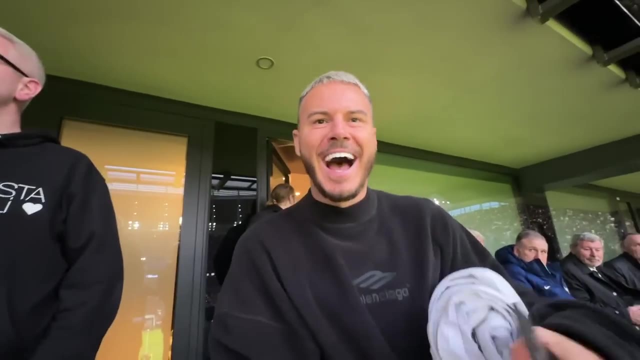 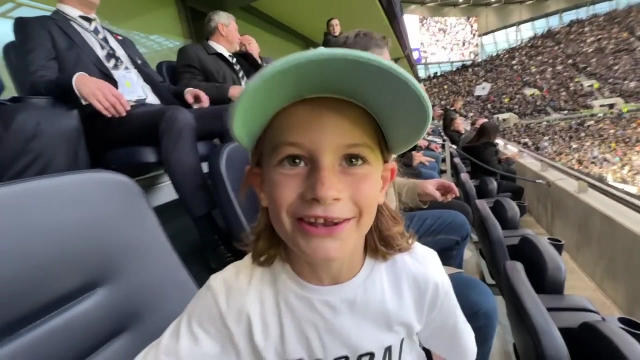 Spurs: 2-1.. Look at him, Look at him. Come on, you Spurs, Come on, Give us your score prediction today. I'm going 2-2.. How are we doing, bro? Score today: 3-1 to Tottenham. 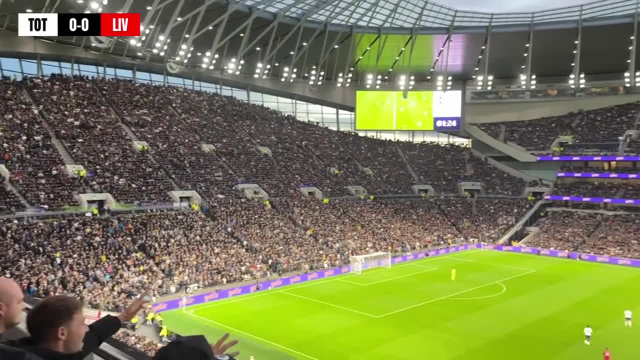 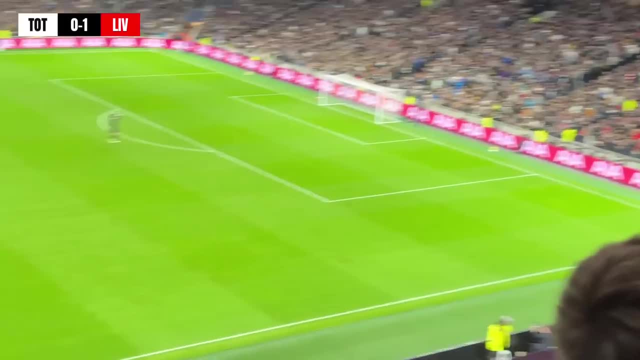 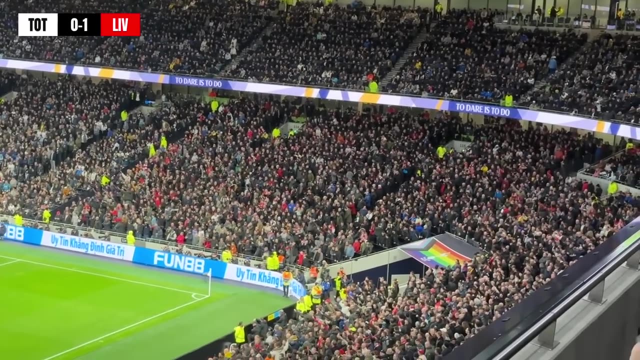 Liverpool kick-off, Liverpool kick-off, Liverpool kick-off. Yeah, Liverpool 1-0 up. Dad, Mo Salah is sensational. The Liverpool fans are loving it. First goal from Liverpool, It's all Liverpool. Liverpool kick-off, Liverpool win. 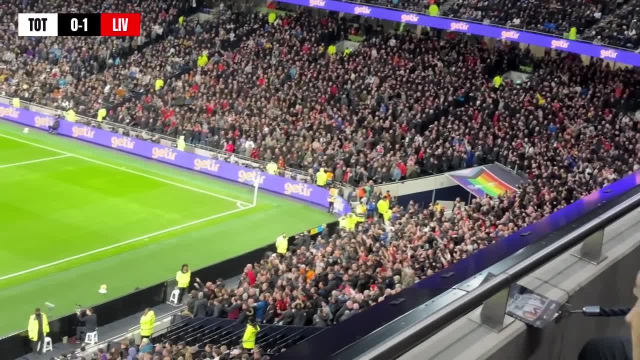 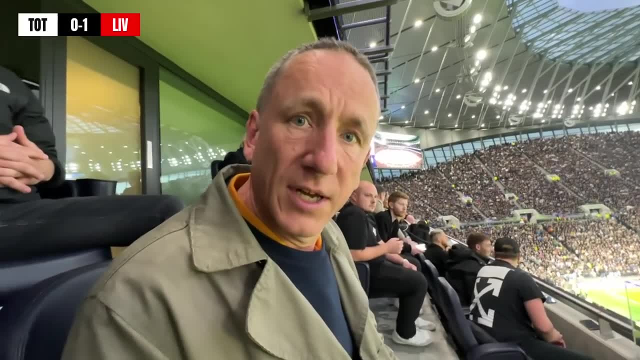 They have it set: Liverpool, Liverpool, Liverpool, Liverpool, Liverpool, Liverpool. I can't give that man an inch of space. He's just too good. Mo Salah is my player in FPL, Yeah, And he's got to give me some points there. 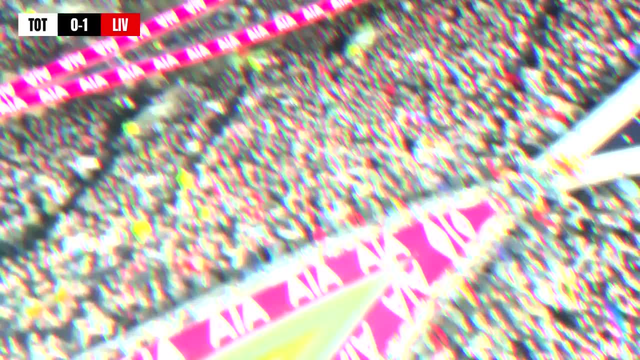 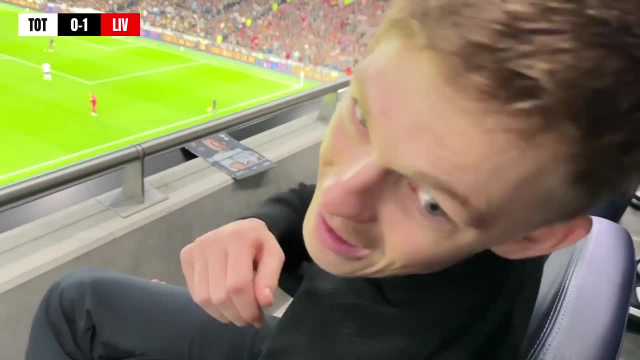 And they gave him too much respect, too much space, So he's going to be punished. Yeah, Liverpool, Liverpool, Liverpool, Liverpool fans loving it. So you're a Tottenham fan. Yeah, I never knew And I'm very, very. 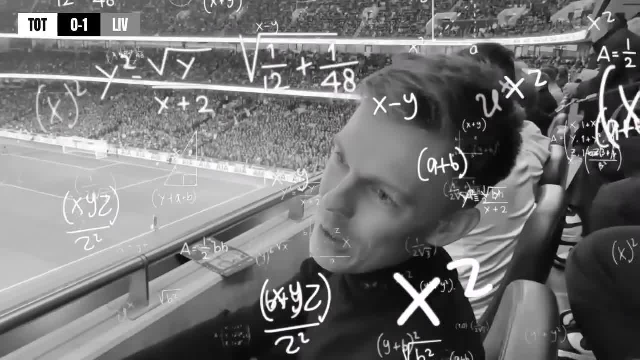 I think it could be a good game. Yeah, I'm very sad that we hit the first there. 3-1 Spurs, It's all being left in 1-1.. You know, just leave the hole. There wasn't enough though. 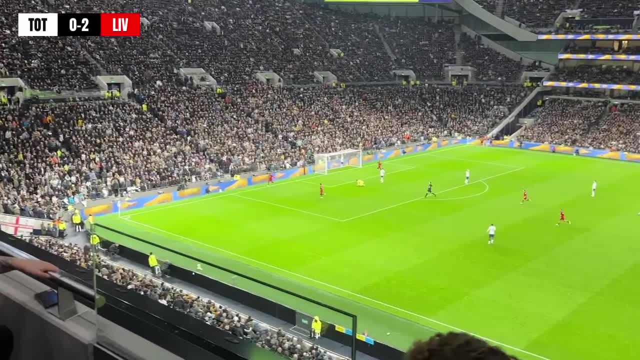 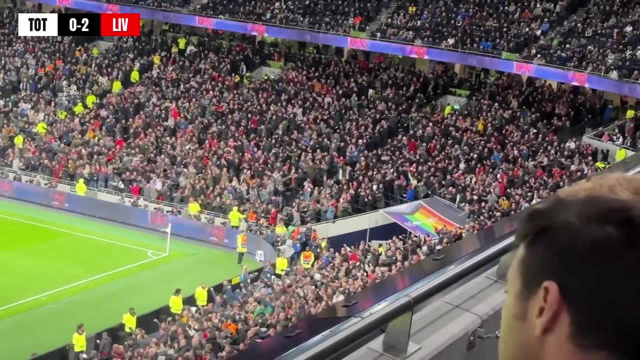 That's not a penalty. Oh no, Mo Salah. That is disgusting. That is absolutely disgusting. He's too good. Liverpool, Liverpool fans. go wild. 40th minute. How do you describe that? You just cannot do that. 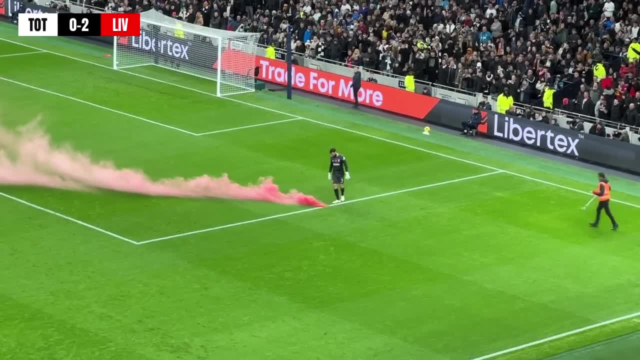 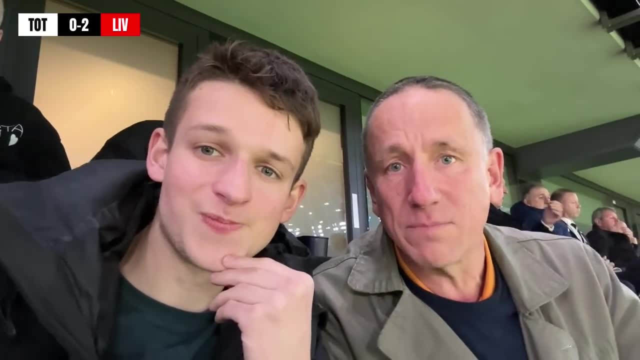 You cannot give him a gift like that. Alisson's going over, He's doing it Top of the hill. Liverpool 2. Mohamed Salah showing his class before the World Cup. Very, very simple: Two chances, two goals. You cannot do that with Mo Salah. 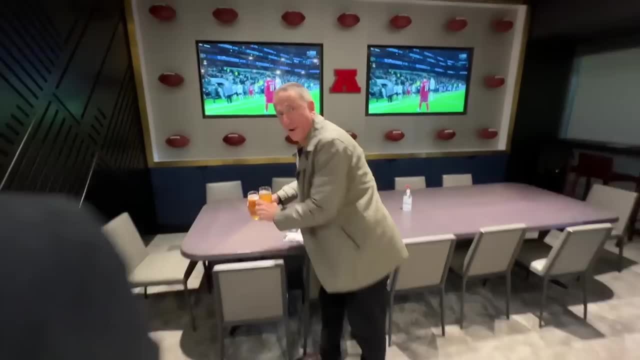 You can't give him gifts like that. What's the time for? Time for a beer? What is this? I don't know whose these are, but let's have one Half time, then. That's what a Liverpool football club are all about. 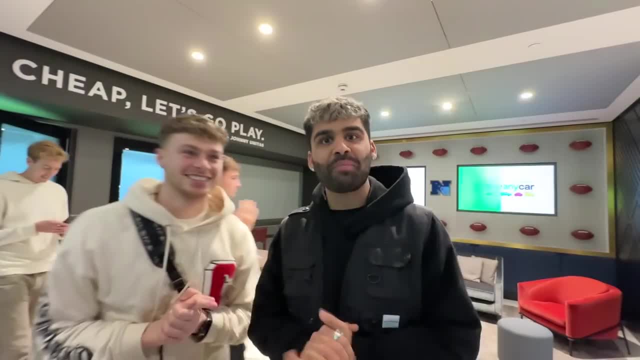 Is that your Liverpool fan? I am. I am indeed. You must be loving it. I'm loving it. I'm really happy. It's a good game. It's going to be a really good game in the second half. A really good game. 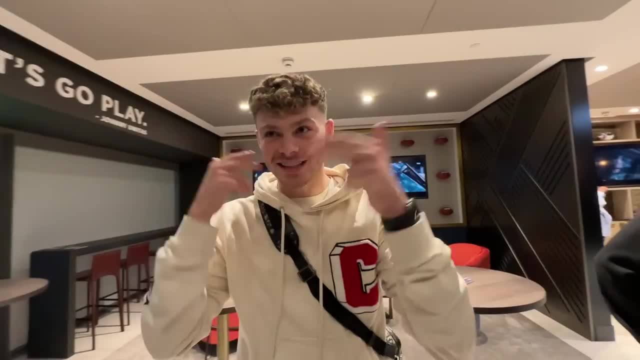 You're fuming. We have to bring him on, don't we? I think we've got to bring him on. I think we've got to chat to the manager. Yeah, yeah, It's so bad that they scored two goals. 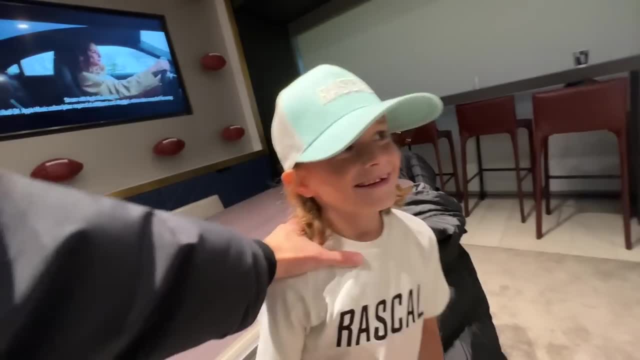 So bad, isn't it? Yeah, We've got to bring him on. We've got to bring you on. Would you come on the second half? Sad face, Sad faces, Sad faces. Mate, do you know what? I've got a hangover. 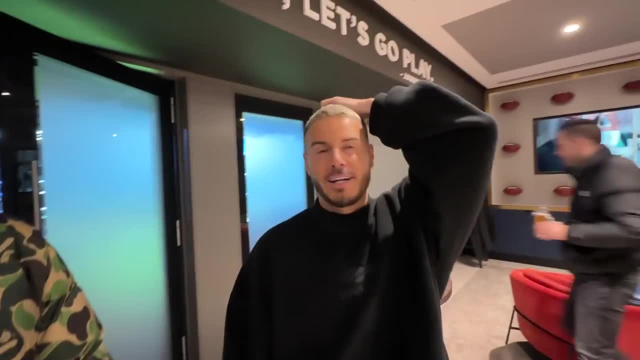 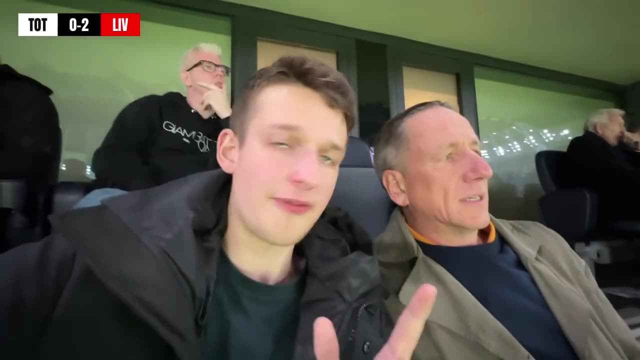 I was out last night. This is just making it worse, Mate. I've got a hangover. I don't even dream Charge for Tottenham. When he comes on, he'll make a difference as well. I've no idea, Theo. 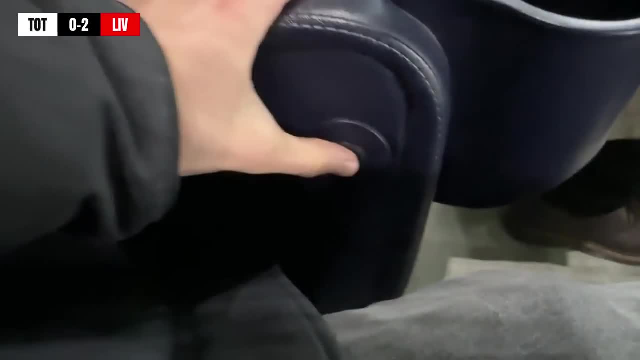 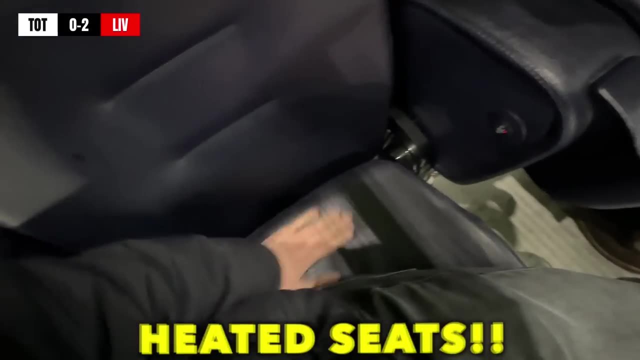 It heats the seat. Oh right, I'm being serious. Look, Look, you see that red thing come up. This seat has now been heated- Heated seats. I've never seen that at a football match, ever. I mean, why is this even needed? 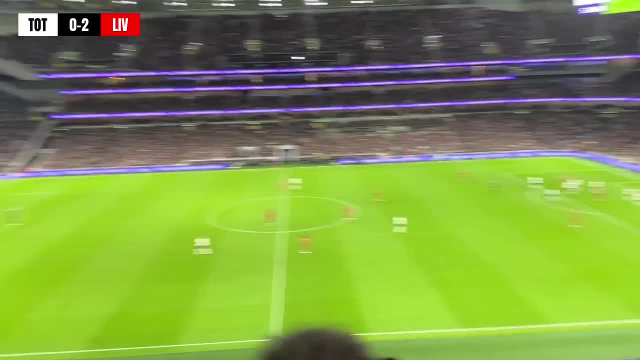 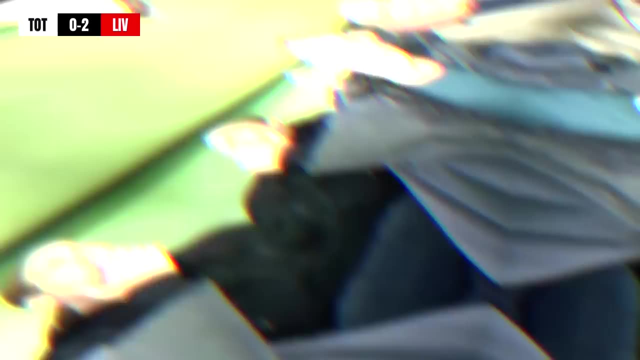 Lovely heated seat in the cold. Salivary's hat trick. Chance for a hat trick. Oh skippy, Oh wow, And he's still on the ball. Ben Tenko is a joke of a footballer. He's a good football player. 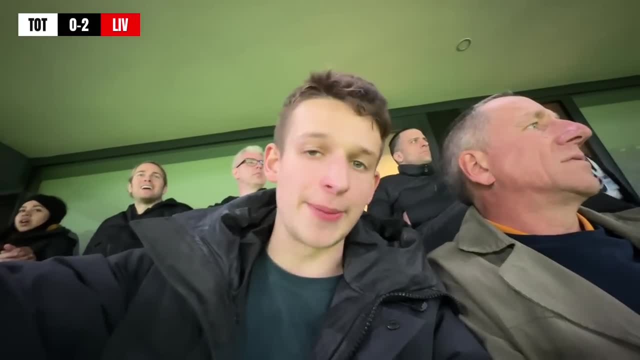 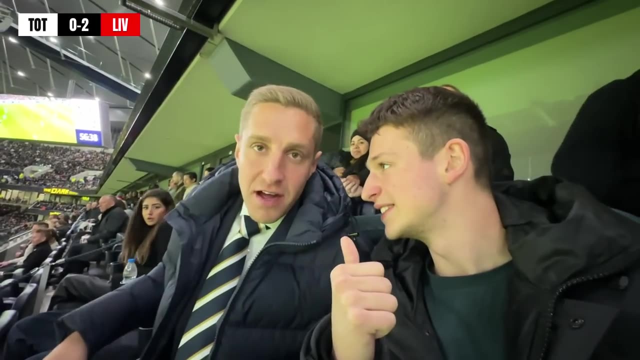 Mate. even against Marseille, they didn't have many forwards. They pushed him into a more attacking position. His close control of the ball was a joke, And we've got a very special guest here. How are we doing Good? I've been bad. 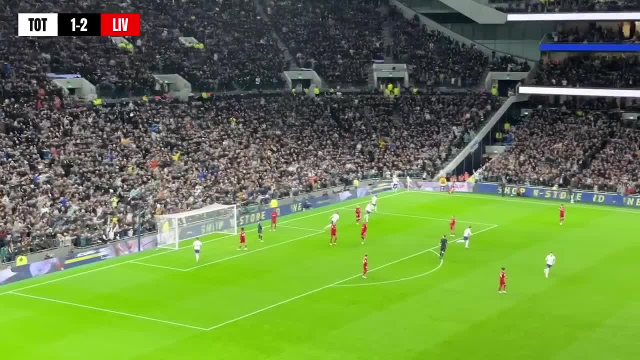 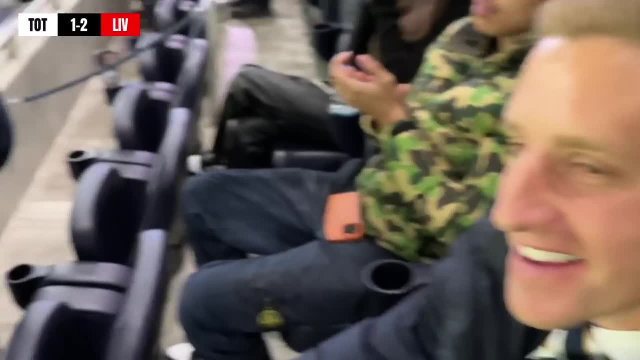 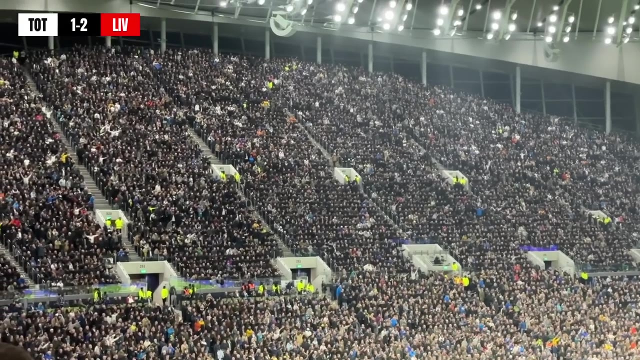 Really, Yeah, We've got a great result. He's going back. He's going back. There. it is One more, One more. Very good finish. It's still tight in front of the goal. I tell you what this is turning into: a classy game. 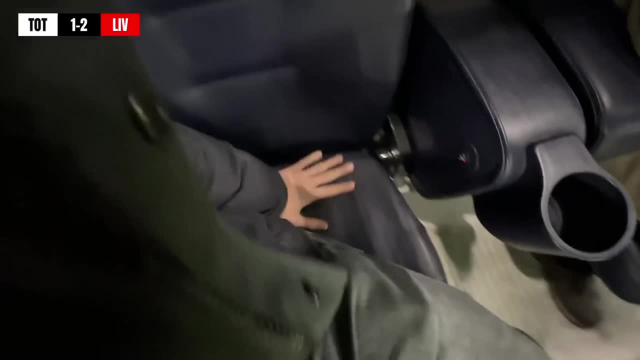 Kulisavsky made all the difference. I said before the match: 3-2.. This heat on here, I can't describe how It's hot, isn't it? It's beautiful mate. Paris 6 with the ball in. 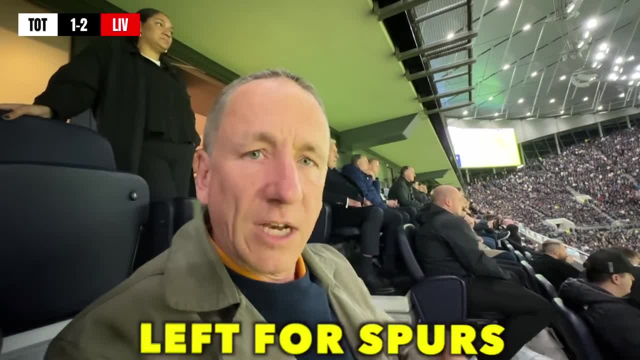 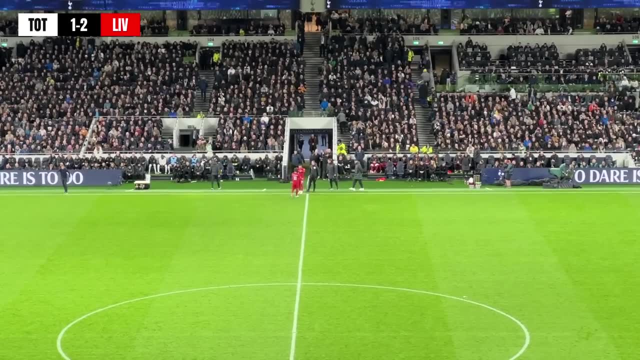 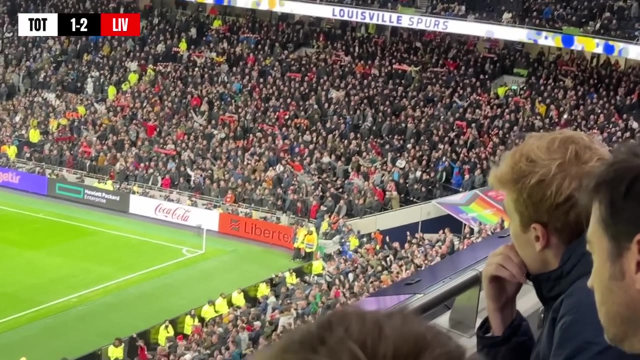 Oh, it's a free header as well. I think it's probably one big chance left for Spurs. That is the big chance. Honestly, Tottenham will look at this game and think: how did we get nothing out of it? Full-time. 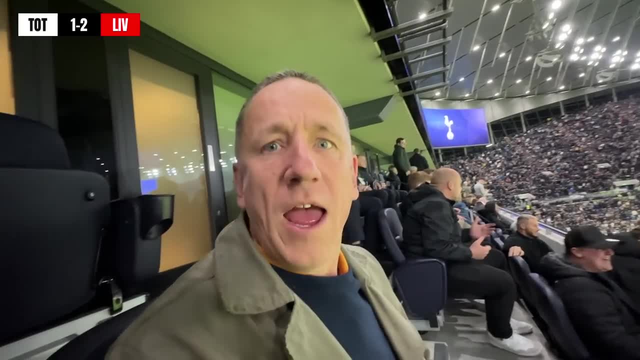 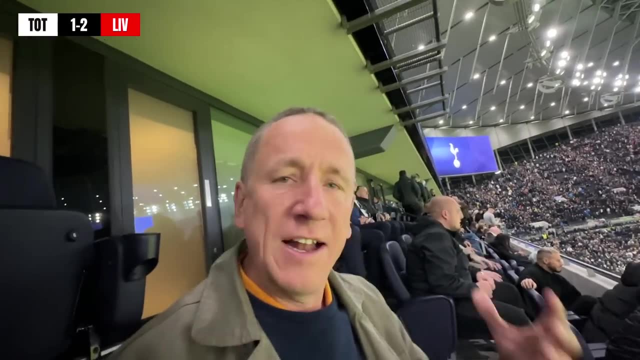 Liverpool take all three points. What an amazing game. Dino In an incredible box, heated seats, but more than that, the football was sensational. Mo Salah was amazing. Tottenham fought back in the second half and was surrounded by YouTubers. 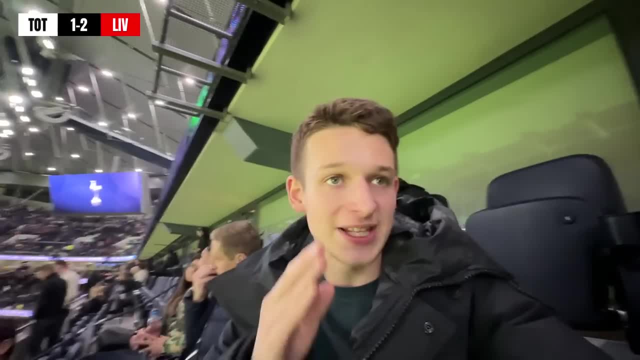 And footballers, ex-footballers, you know everything. It's amazing, We have to say. this is probably the best seat I've ever been in. Glass of wine, a bit of NFL. Is that going in there now? Yeah, you'll see later. And he just: 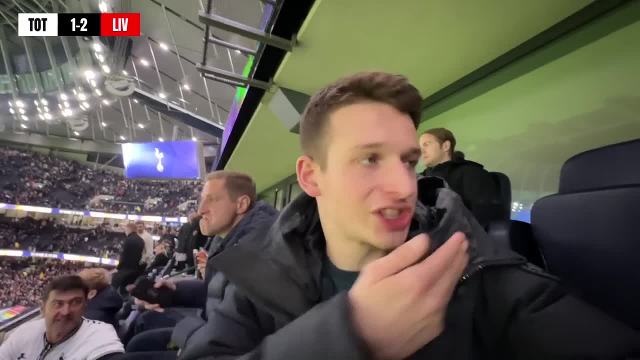 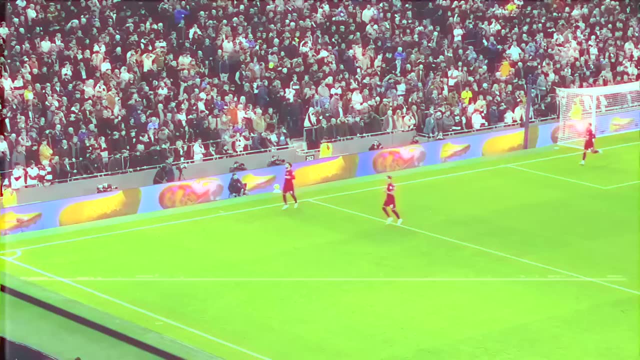 has to walk in there Before the match. you're there for an hour. two hours After the match, you're in there. That's the special fitness that you pay for. Mo Salah masterclass. The football was great. The seats were even better In terms of comfortable VIP private feel. it's just the. 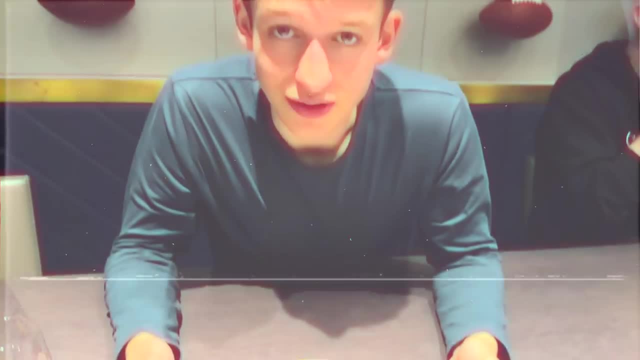 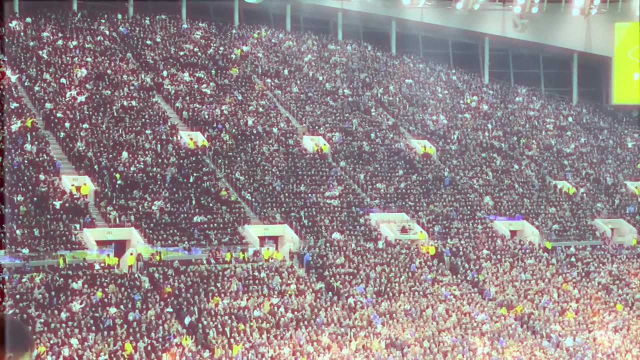 best. The food was immaculate. It felt like I wasn't in a stadium. It felt like restaurant food or home-cooked food. It was that fresh. The one billion pound investment was definitely worth it. I'll be real, though: If you're going to a football match, for Atmosphere, this ain't the place, Billy. 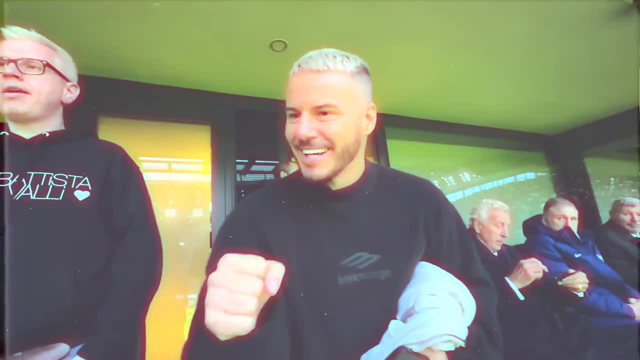 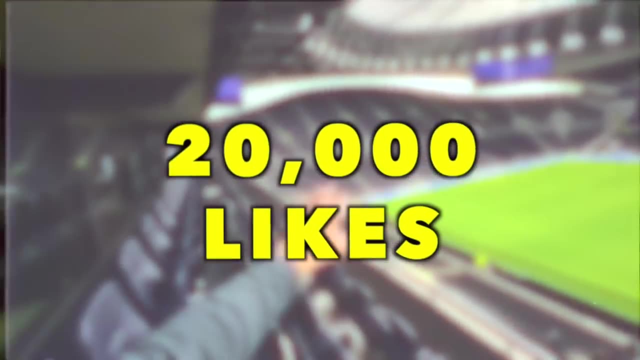 Wingrove, Roman the father-son duo, second best on YouTube in my opinion. The South African boys, everybody in there was top class 20k likes and I will do the cheapest version in the Premier League And I bet you it will be better for Atmosphere, That's guaranteed And it's been. 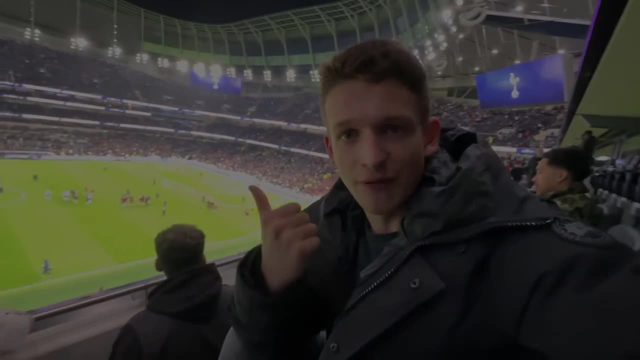 a pleasure to sit in the best seat in the house. What was a great game of football.